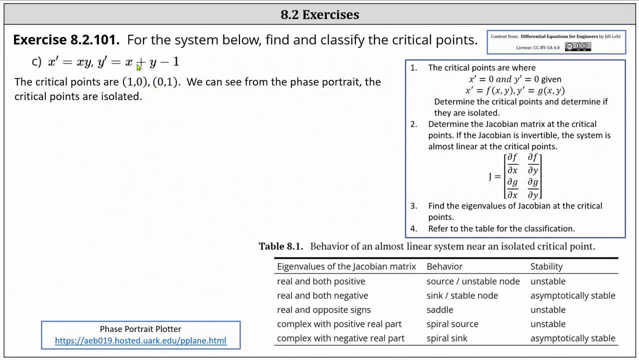 there are no other x and y values where both x prime and y prime are zero near these two points, which indicate the critical point is zero. So the critical points are isolated. Let's also verify this by looking at the corresponding vector field as well as the face portrait. We'll do this using the online tool referenced below. 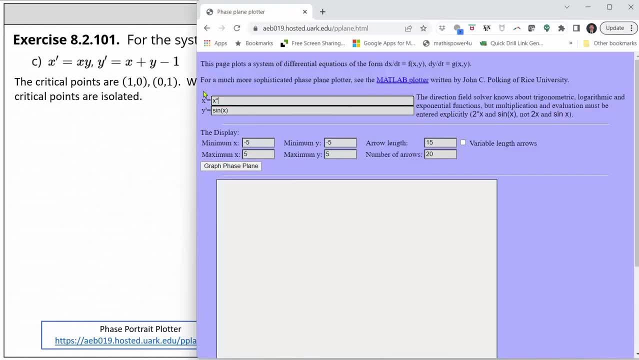 We begin by entering the equations We have: x prime equals x times y tab. y prime equals x plus y minus one. Let's also change the display, Let's change the window so both the x and y axes go from negative two to positive two. 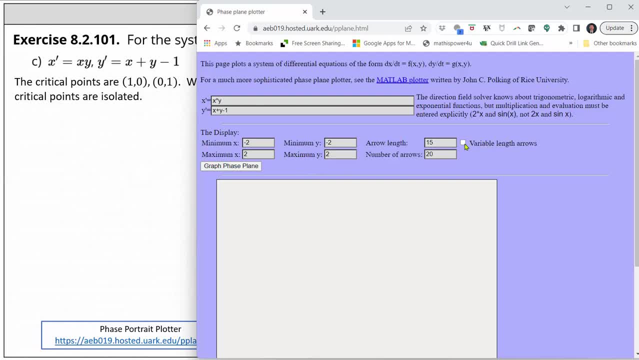 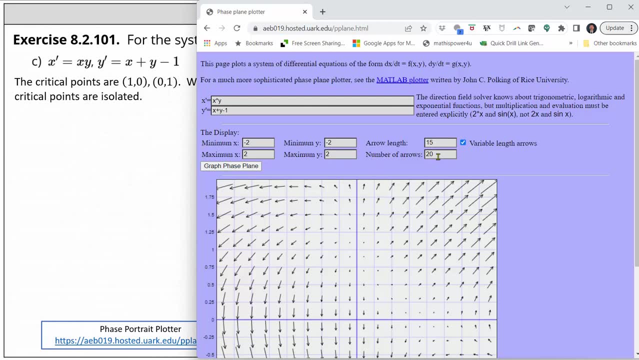 Let's also click on the box variable length arrows on the right and now click graph. We can change the density of the vector field by changing the number of arrows and we can change the scaling of the vectors by changing the number for arrow length. 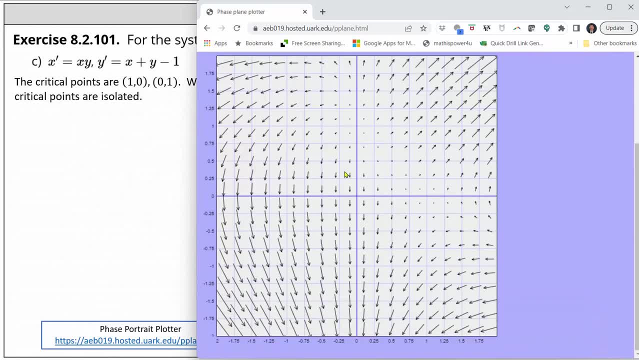 But this looks pretty good. Let's scroll down. The vector field does verify. we have a critical point at one comma zero, which is here, as well as zero comma one, which is here. Recall: this is where both x prime and y prime are zero. 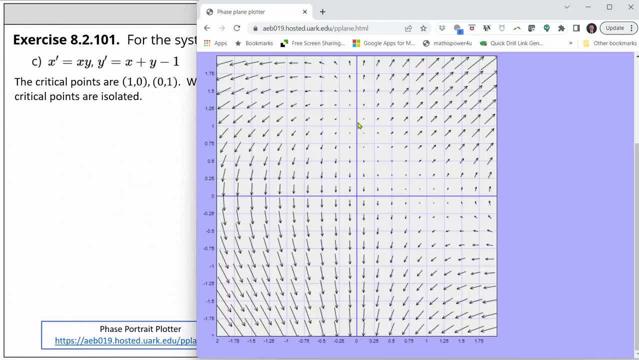 Which means we'd have a zero vector in the vector field. And also, if we zoom in near those critical points, we don't have any other critical points, which again verifies the critical points are isolated. To emphasize this even more, let's sketch some trajectories by clicking on points on the coordinate plane. 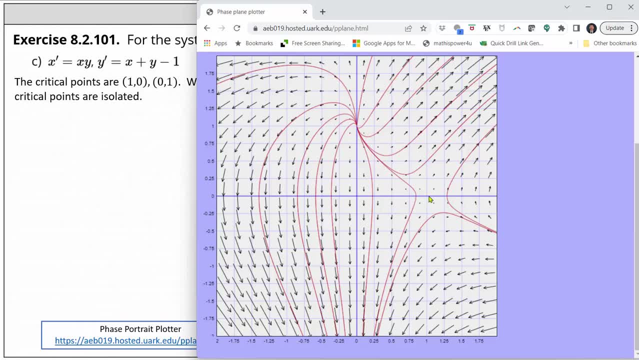 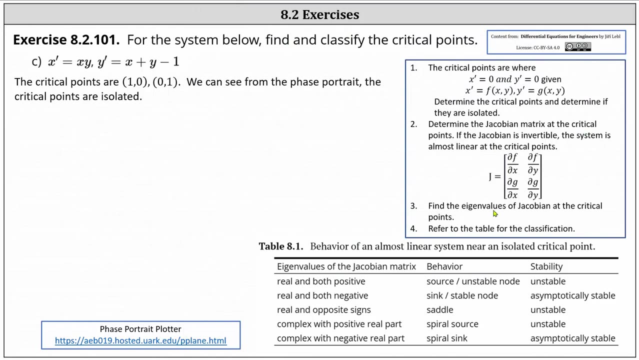 Using the trajectories, it appears the point one, comma zero is a saddle point and the point zero, comma one is a source. Let's go ahead and verify this formally. The next step is to determine the Jacobian matrix at the critical points, and then we determine the eigenvalues of the Jacobian at the critical points. 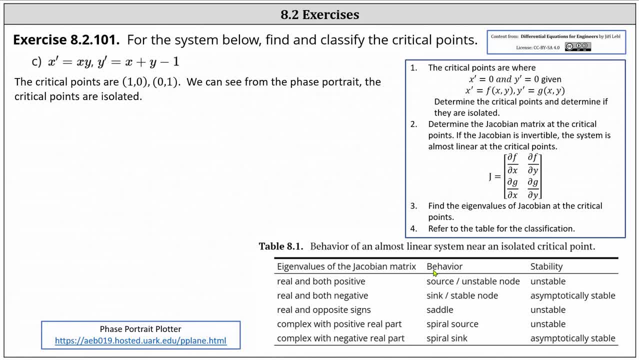 The types of eigenvalues we have determine the behavior as well as the stability at the critical point. So let's work on determining the Jacobian, which is the two by two matrix defined here. where x prime is equal to F of x comma y and y prime is equal to g of x comma y, The partial of 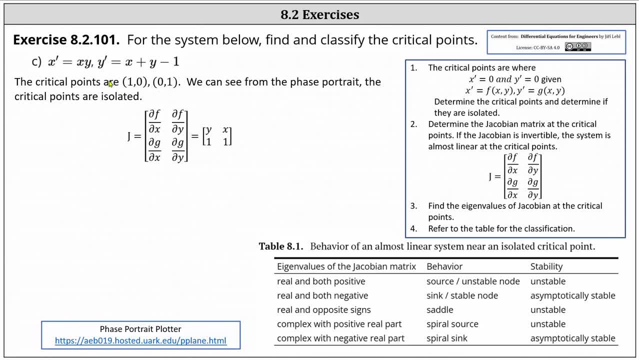 f of the spectre x is the partial of xy with respect to x, which is y. The partial of f of the spectre y is a partial of xy with respect to y, which is x. In the second row we have the partial of g with respect to x, which is the partial of x plus y minus 1, with respect to x, which is 1.. 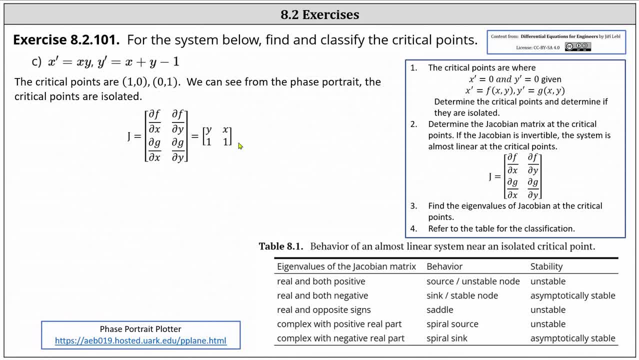 And the partial of g with respect to y is also 1.. And now we determine the Jacobian matrix at at the first critical point of one comma zero. We substitute one for x and zero for y. The Jacobian at one comma zero has entries zero: one one. 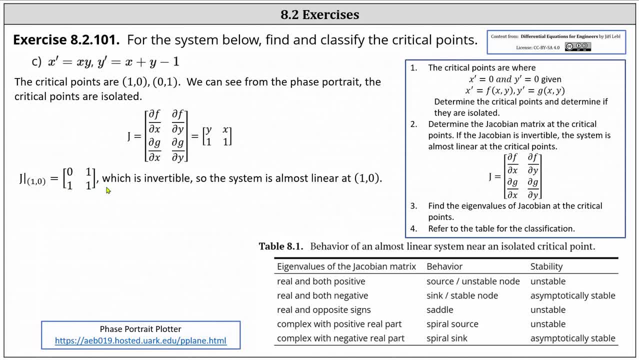 one Notice: this matrix is invertible, meaning it has an inverse because the determinant is not zero. This is in case the system is almost linear. at the critical point, one comma zero. Next we determine the eigenvalues of the Jacobian. To do this, we set up and solve the equation. 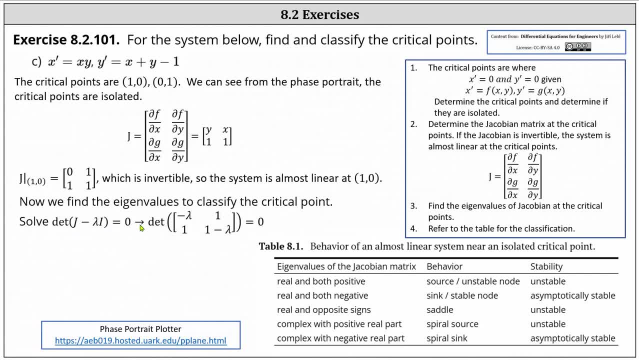 the determinant of the difference of j and lambda i equals zero. The result is the determinant of this two by two matrix equals zero. giving us negative lambda times the quantity one minus lambda minus one equals zero. Solving for lambda, we have negative 1 1⁄2. 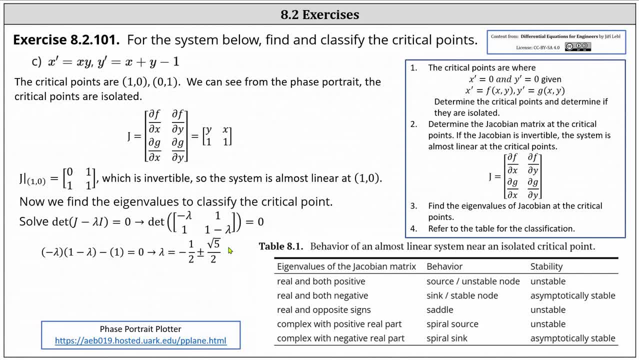 plus or minus square root of five divided by two. Notice we have two real solutions: One is positive and one is negative. If we were to enter our table, because both eigenvalues are real and opposite signs, we have a saddle and the stability is unstable. 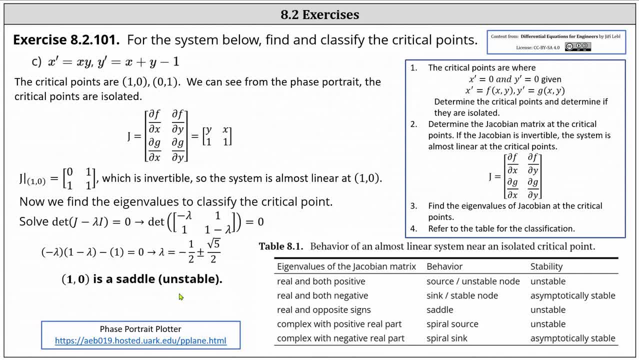 The point one comma zero is a saddle and the stability is unstable. And now we go through the same process for the second critical point of zero comma one. The Jacobian, at zero comma one has entries one, zero one, one which, once again, is invertible. 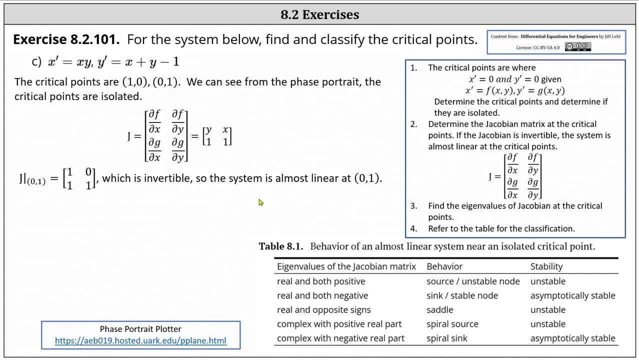 so the system is almost linear at the point zero comma one. And now we determine the eigenvalues of the Jacobian, We set up our determinant, which results in the determinant of this two by two matrix equals zero. This gives us the equation. 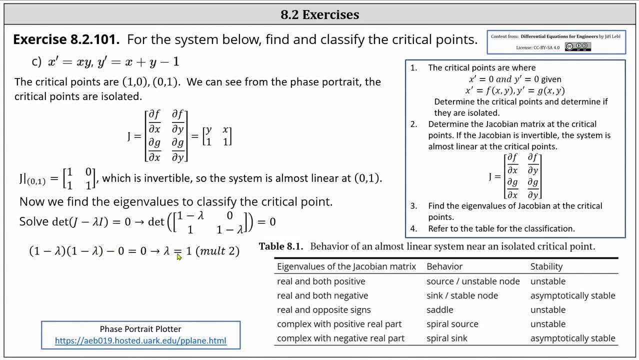 the square of one minus lambda equals zero and therefore lambda equals one which has multiplicity two. Therefore, we treat this as two real positive eigenvalues which, again referring to our table, indicates: at the critical point zero comma one, we have a source or unstable node. 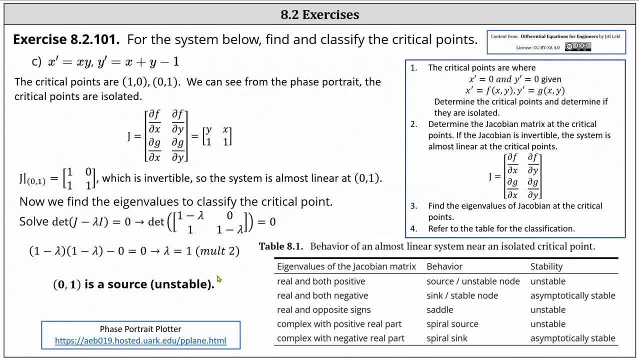 and the stability is unstable. Going back to the phase portrait one last time: we have a source or unstable node and the stability is unstable. Going back to the phase portrait one last time: we have a source or unstable node and the stability is unstable. 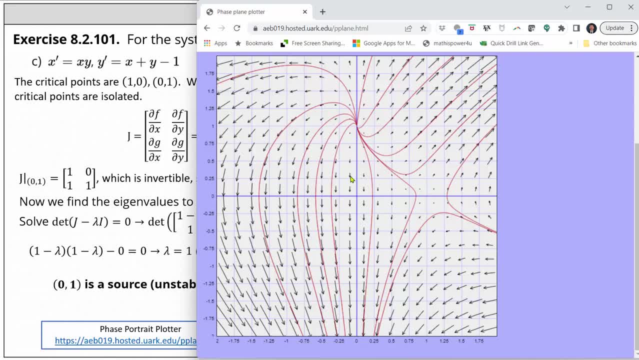 The phase portrait does support our findings. I hope you found this helpful.